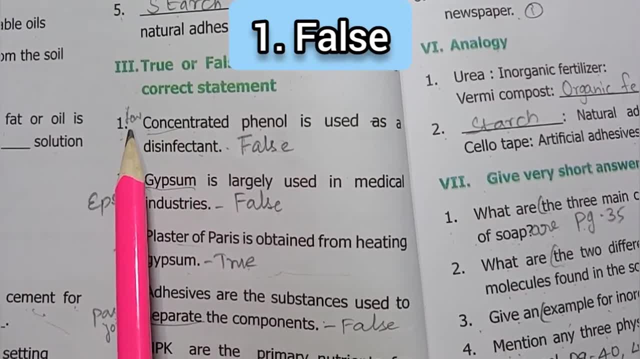 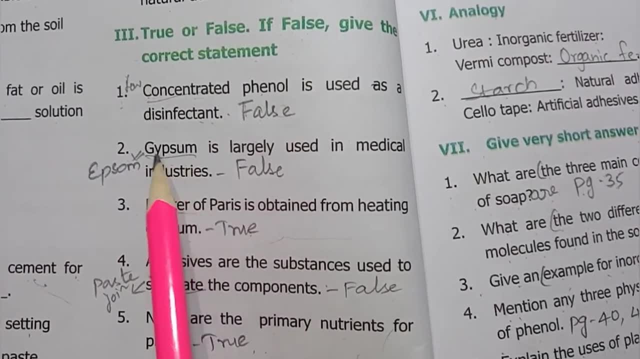 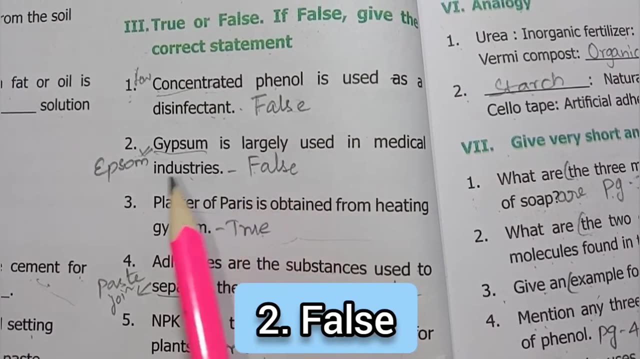 The answer is false. What is the correct statement? Low concentration. This is high concentrated, In that low concentrated phenol is the disinfectant. Then second one: Gypsum is largely used in medical industries. False. The correct statement is: gypsum is not used much in medical industries. 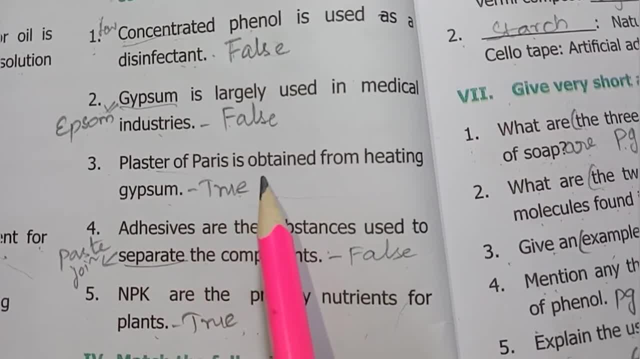 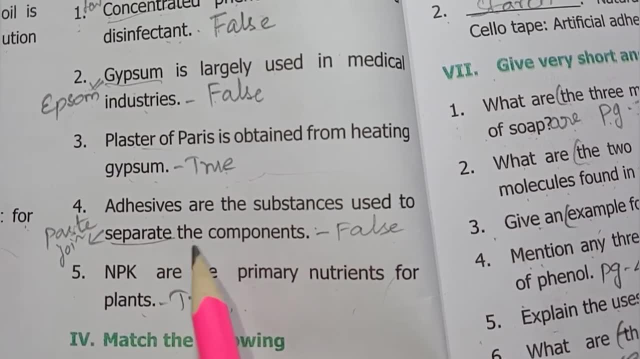 Epsom. Third one: Plaster of Paris is obtained from heating gypsum- True. Fourth one: Adhesives or the substances used to separate the components- False. The correct statement is: adhesives are used to paste, to join. 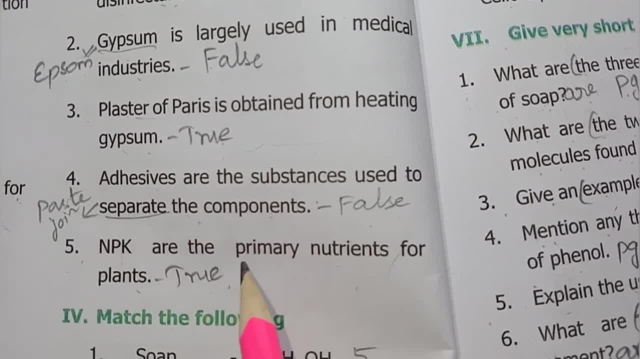 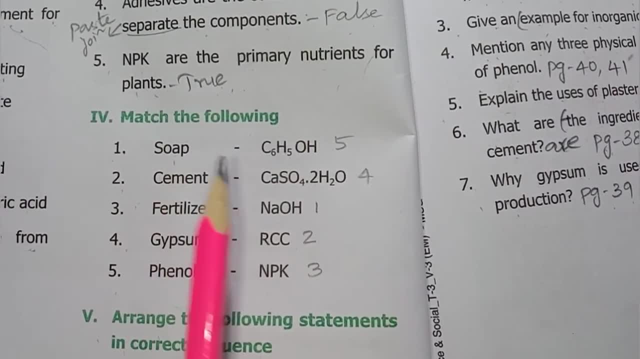 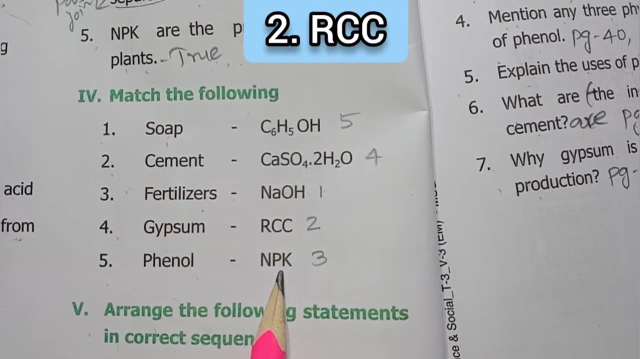 Not to separate. Then, fifth one, NPK, or the primary nutrients for plants. True, Then Roman letter 3.. Match the components: First one, Soap, NaOH. Second one Cement, RCC. Third one Fertilizers NPK. 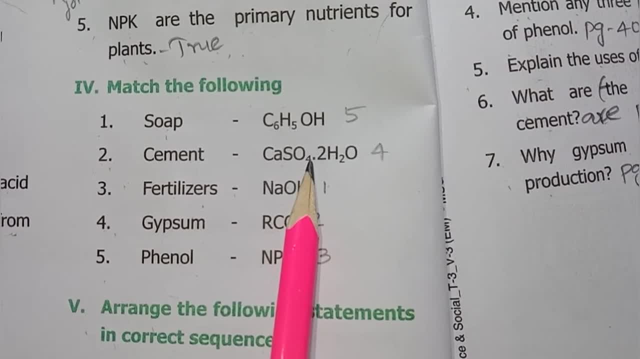 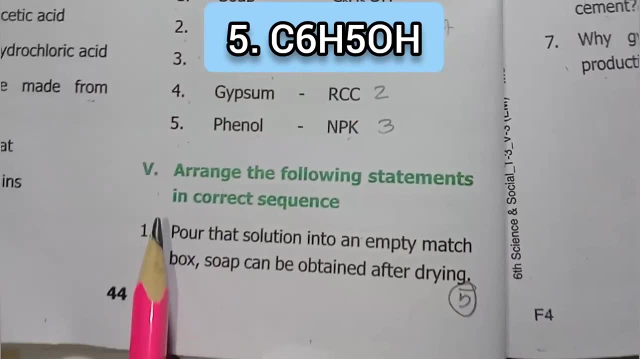 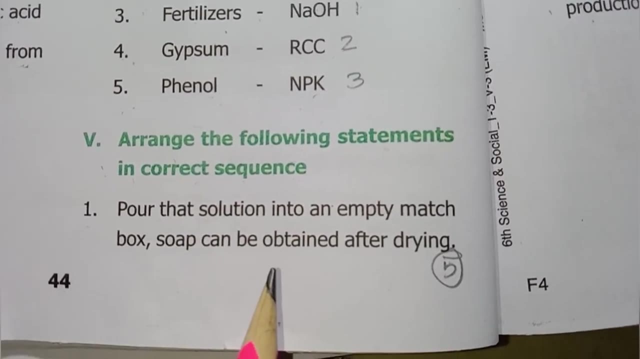 Fourth one: Gypsum CasO4.2H2O, Then phenol C6H5OH, Then Roman letter 5.. Arrange the following statements in correct sequence. So six points are given. Arrange in correct sequence, So first one is. 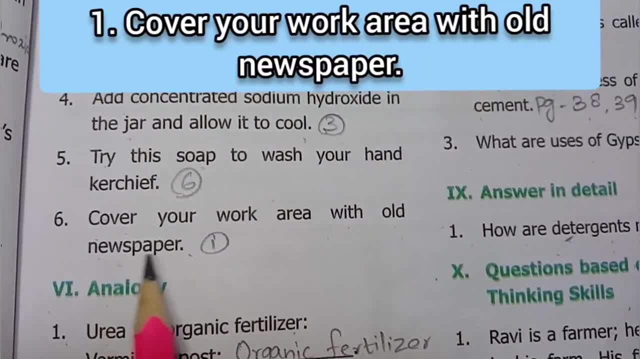 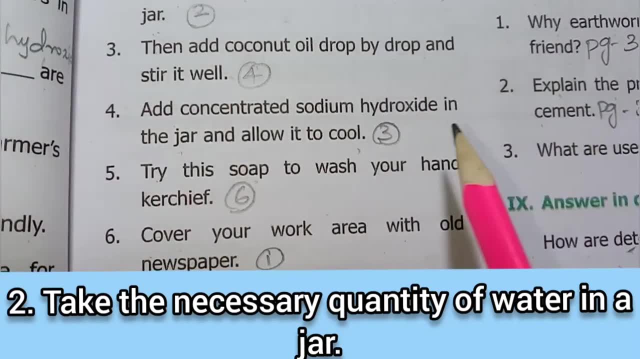 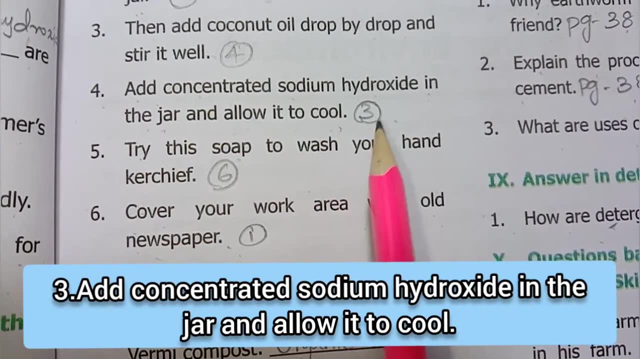 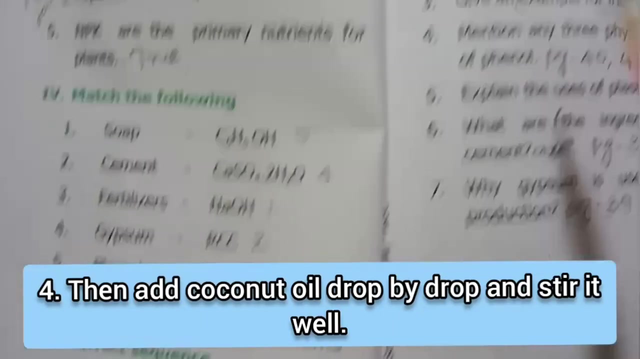 Close your mouth. Next point is: Cover your work area with old newspaper. Then second one second point: Take necessary quantity of water in your jar. Third one is Fourth point is Four concentrated sodium hydroxide in the jar and allow it to cool. 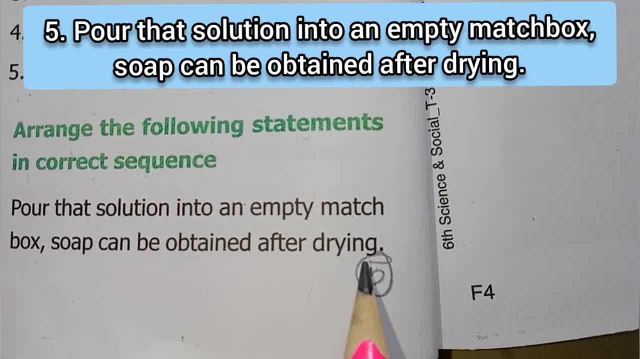 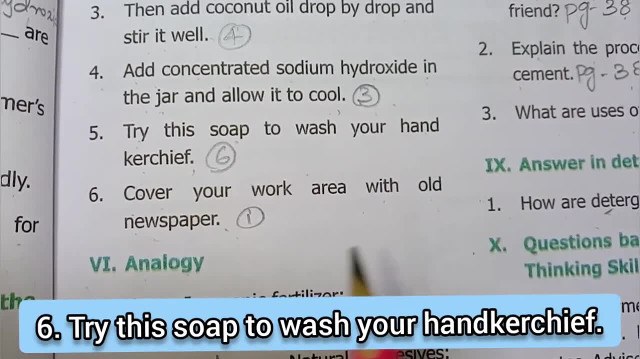 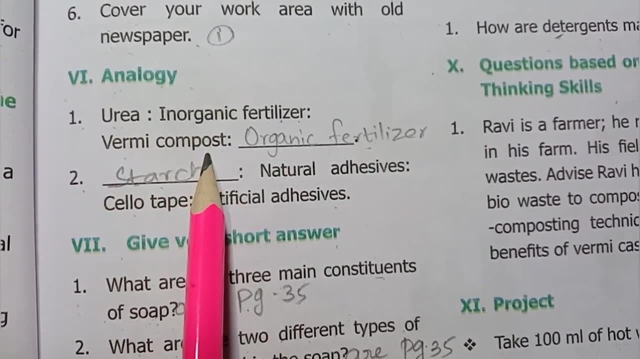 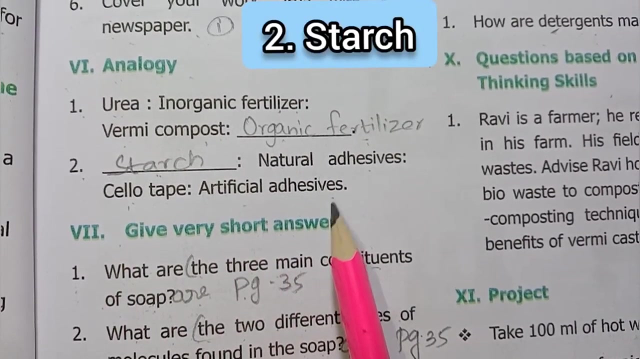 Fourth, one Third point: Soap can be obtained after drying. sixth point. on the fifth point, try the soap to wash your handkerchief. okay then Roman letter 6, enology, urea, inorganic fertilizer, vermicompost organic fertilizer, starch, natural adhesives, cellotape, artificial adhesives. so answer is: first one organic fertilizer, second, one starch. 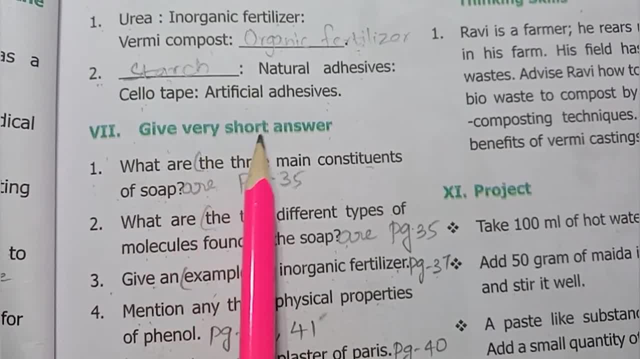 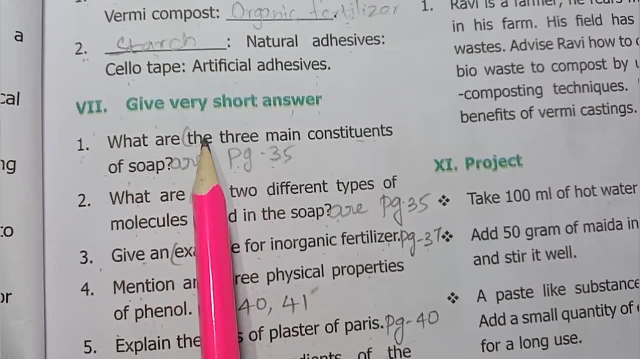 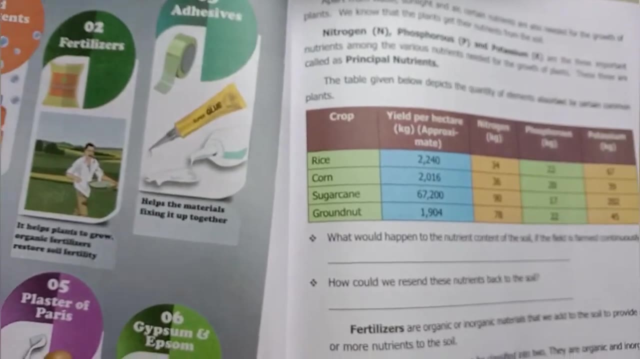 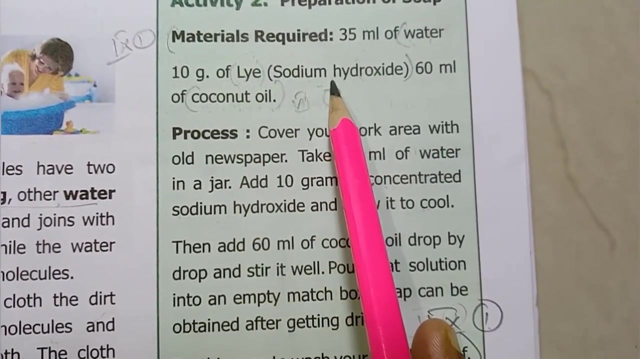 then Roman letter 7, give very short answer. first one: what are the three main constituents of soap? page number 35,, that is write from the question. the three main constituents of soap are page number 35,, 35, in this box see water, lye, sodium, hydroxide coconut oil. these are the four points: water, lye, sodium, hydroxide coconut oil. 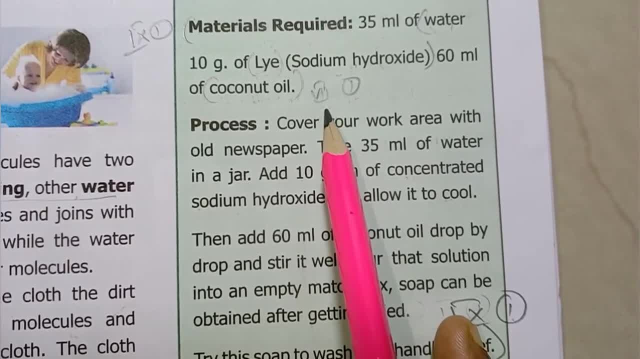 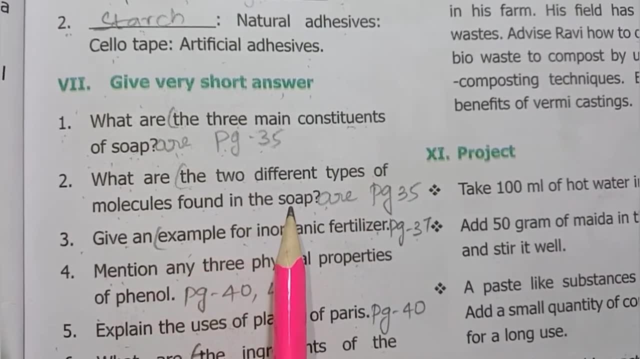 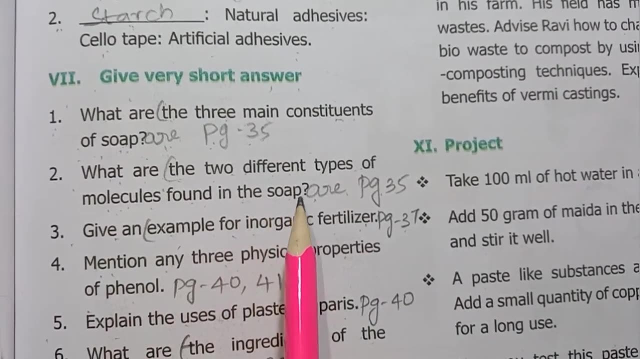 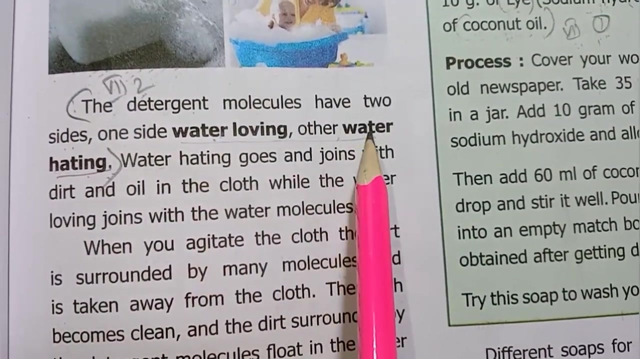 hydroxide coconut oil. seventh Roman letter. first one can answer, then second one: what are the two different types of molecules found in the soap, page number 35,. if you write from the question, the two different types of molecules found in the soap are: write the same, page, number 35,. see here in this paragraph, water loving, water hating. water loving and water hating. if you write from the question. if not, 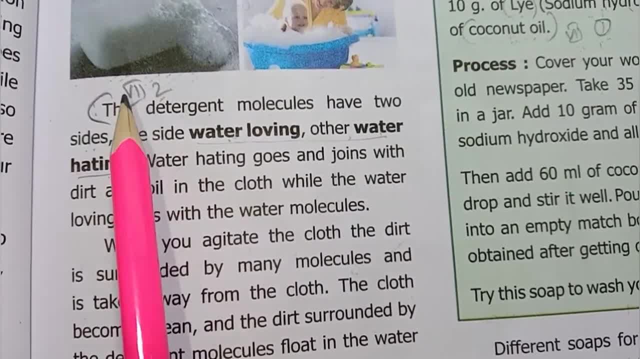 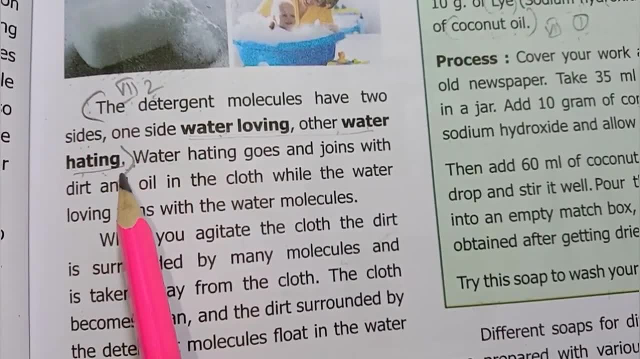 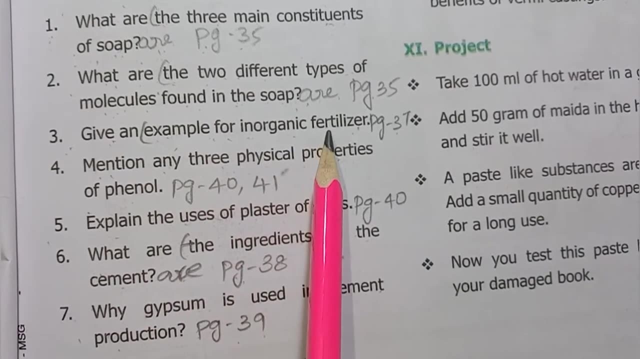 start from the detergent molecules. water hating close with detergent and water hating. seventh Roman letter, second one. if you write from the question water loving and water hating, if not start from here and water hating with 7th Roman letter, second one, then third one. give an example for inorganic fertilizer, page number 37, inorganic fertilizer example. 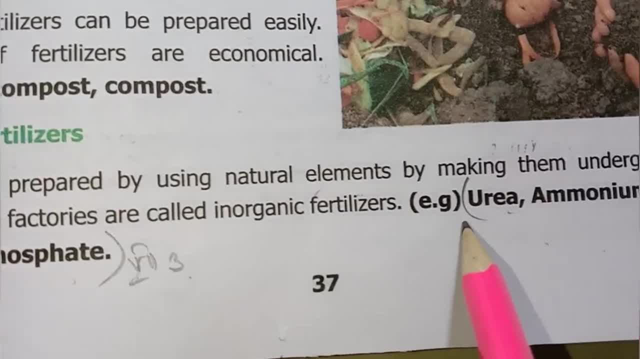 page number 37, inorganic fertilizer paragraph in 8th chapter, urea, ammonium, sulfate and oxalate- that is new Michelin star- And superphosphate, 7th room, letter 3rd. one can answer. 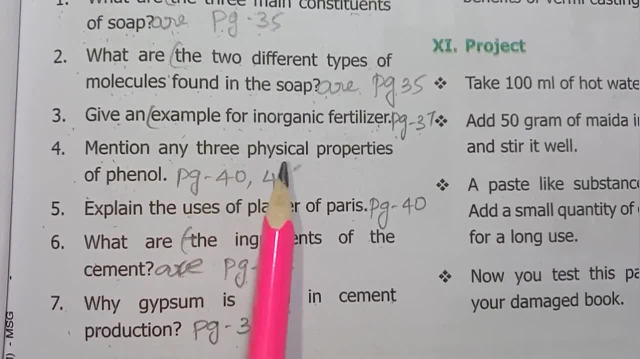 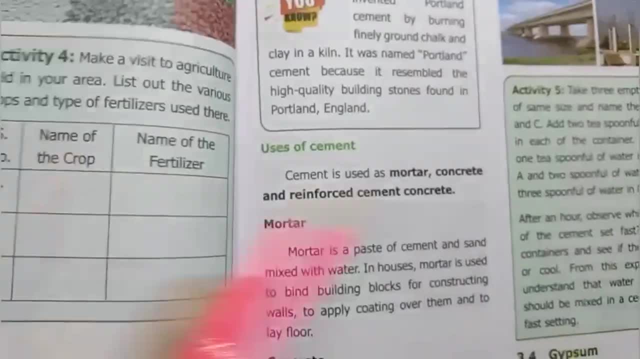 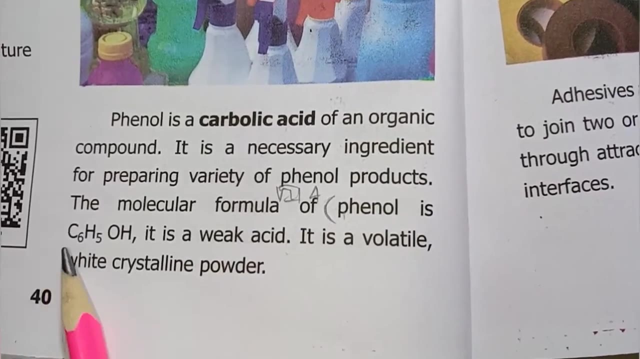 Then 4th one Mention, any 3 physical properties of phenol, Page number 40 and 41.. The phenol in the drawing, Phenol, paragraph 3, physical properties. So phenol is C6H5OH. It is a weak acid. 1 point. 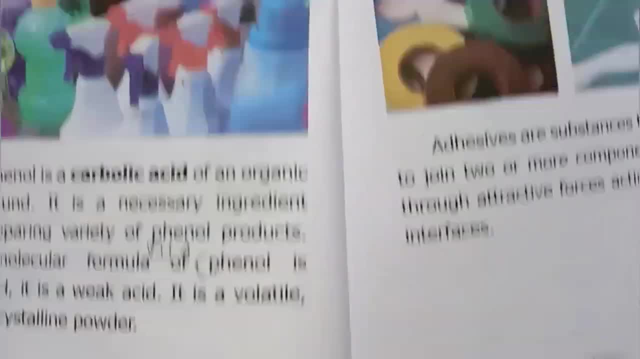 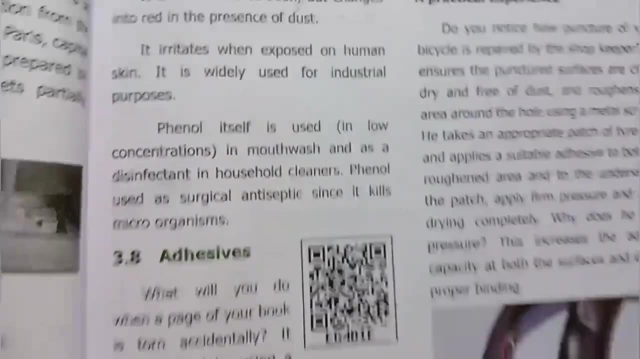 It is volatile, While crystalline powder- 2nd point- Then it is a colorless solution. Close with that, 7th room letter 4th one, 3 points, Then 5th one, Explain the uses of plaster of Paris. 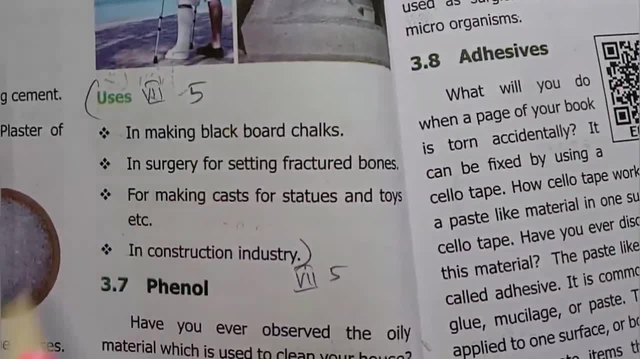 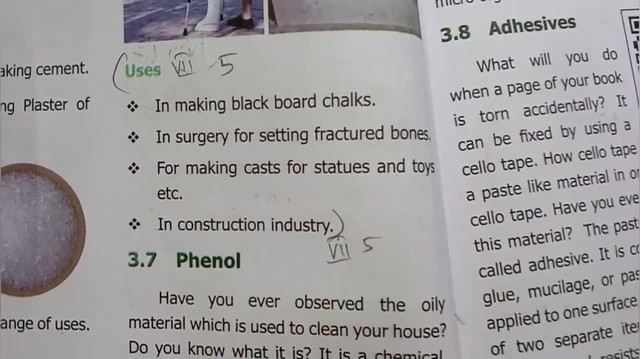 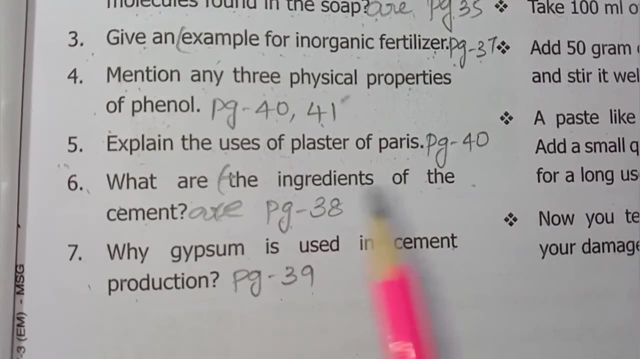 Page number 40. Plaster of Paris uses- See this In making the 4 points. Its uses 7th room, letter 5th. one can answer Then 6th one: What are the ingredients of the cement? 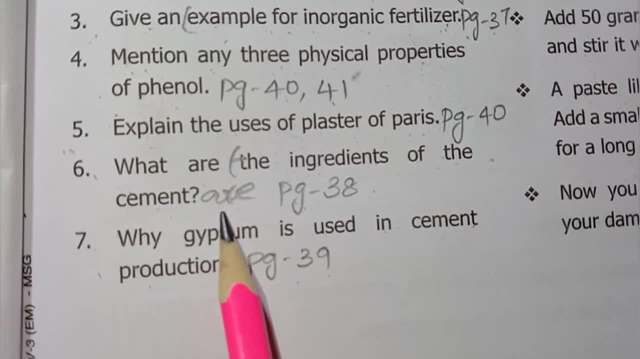 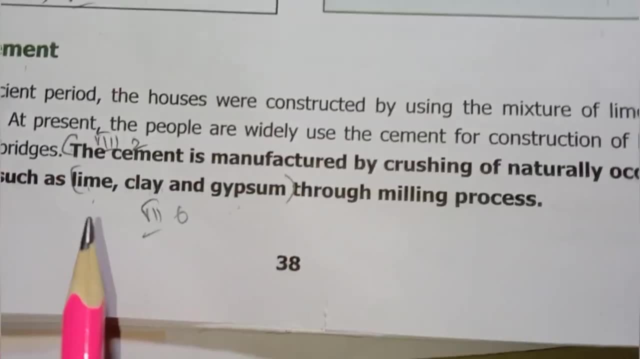 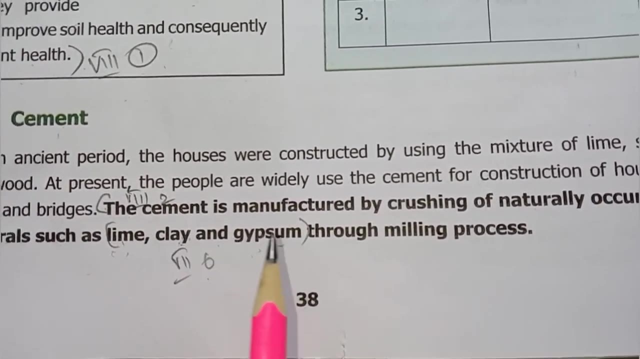 Page number 38.. The ingredients of the cement are Page number 38.. Here it is Lime clay and gypsum. 7th room, letter 6th. one can answer Lime clay and gypsum, Then 7th one. 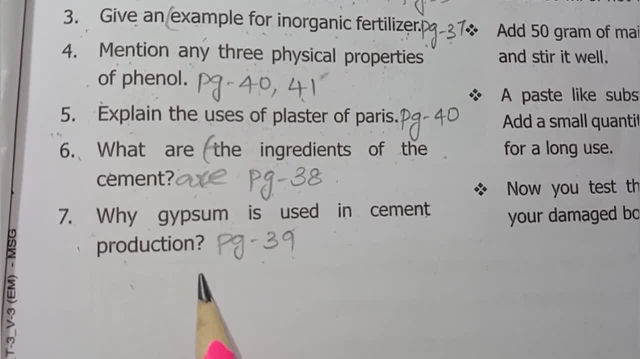 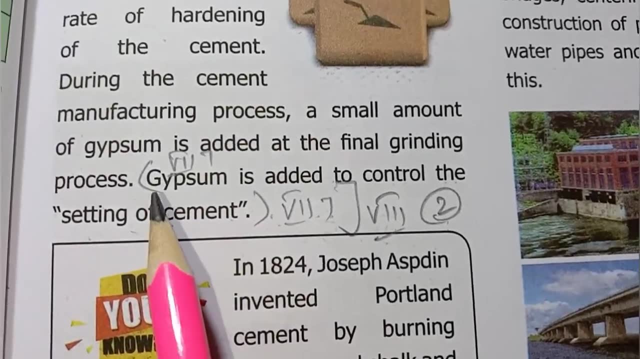 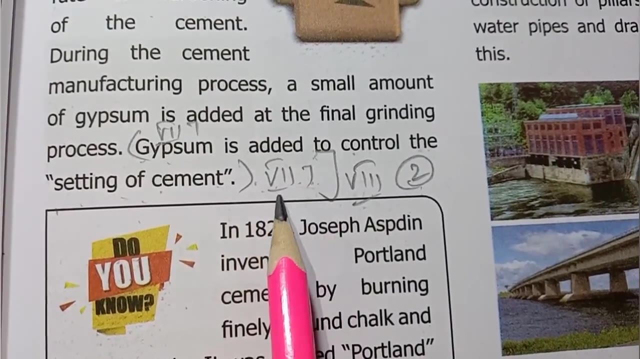 Why gypsum is used in cement production. Page number 6th one. Page number 39.. In the gypsum paragraph- See the last line On the box- Gypsum is added to control the setting of cement. 7th room, letter 7th. one can answer. 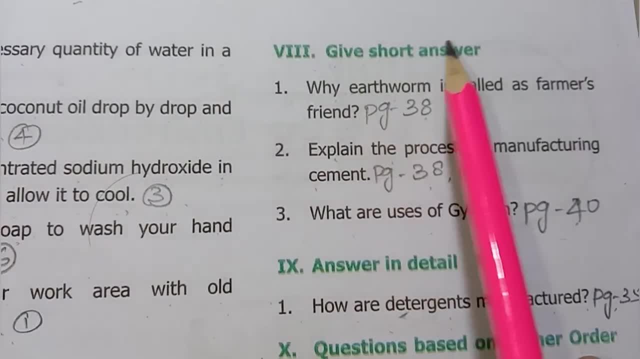 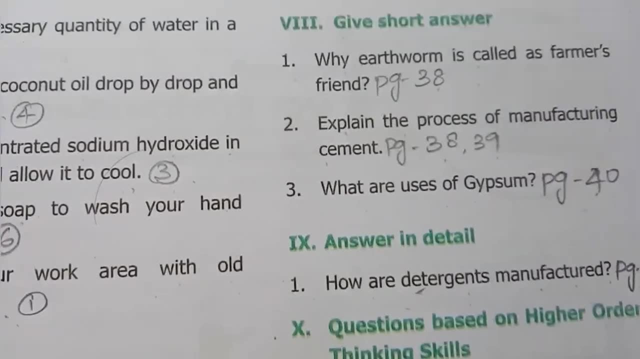 Then Roman letter 8.. Give short answer. First one, Why earthworm is called as farmer's friend. Page number 38.. Page number 38.. Page number 38.. So you can see the box. You can see the box. 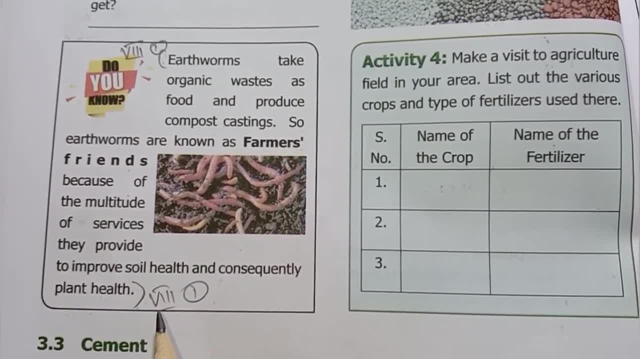 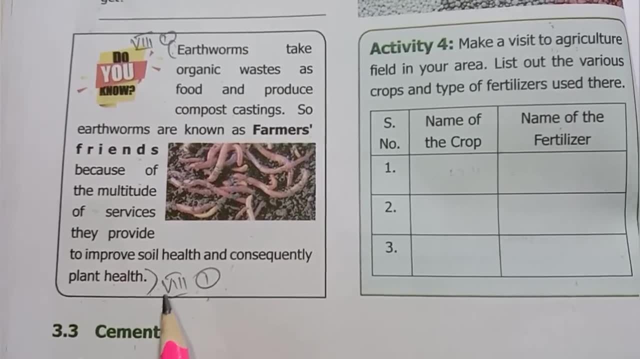 Start with earthworms, Close it with plant health. 8th room, letter, 1st one can answer: Earthworms Stakes. Start with earthworms, The whole one paragraph. 8th room, letter 1st one can answer. 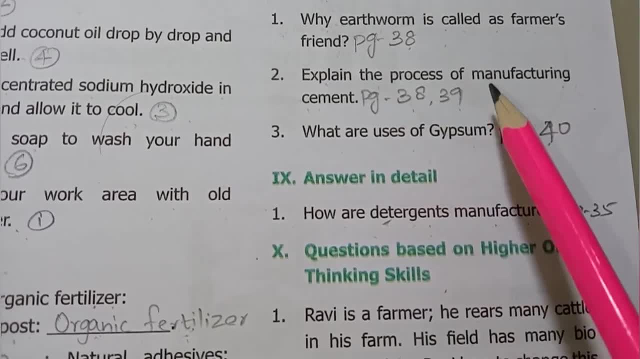 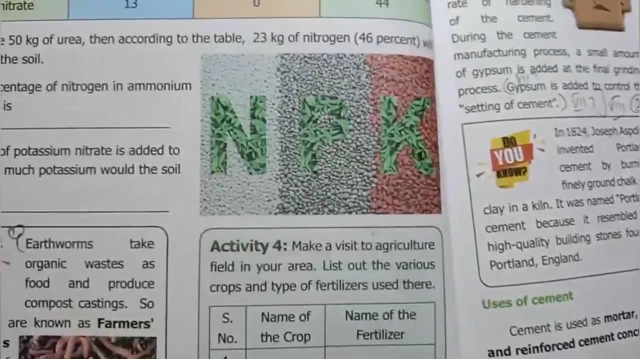 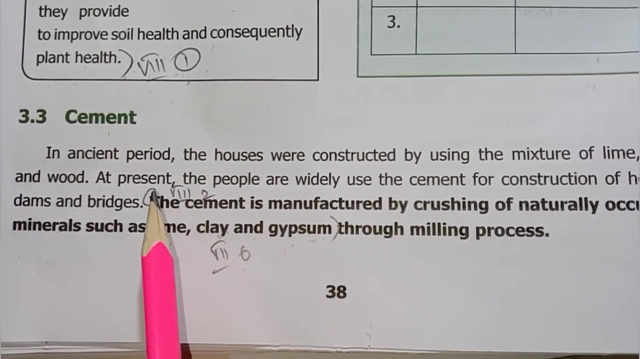 Then, 2nd, one Explain the process of manufacturing cement. Page number 38 and 39.. Page number 38 and 39. Below the cement, paragraph 3rd line, letters. there clear the cement is manufactured. other than this. start paneer pray. next to paragraph, next page, there can and the paragraph for say the 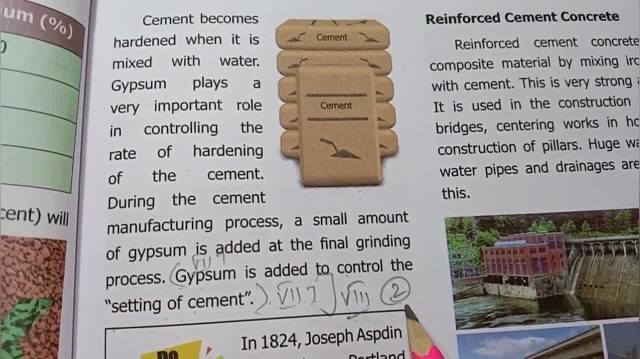 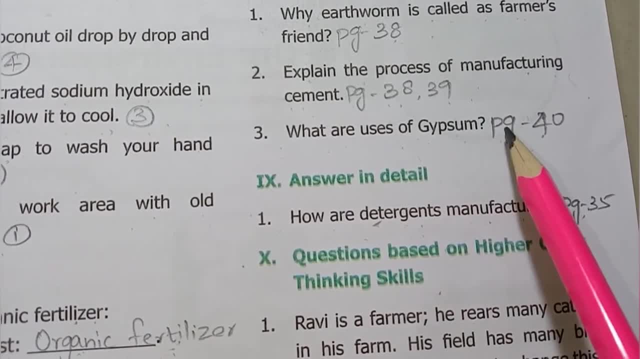 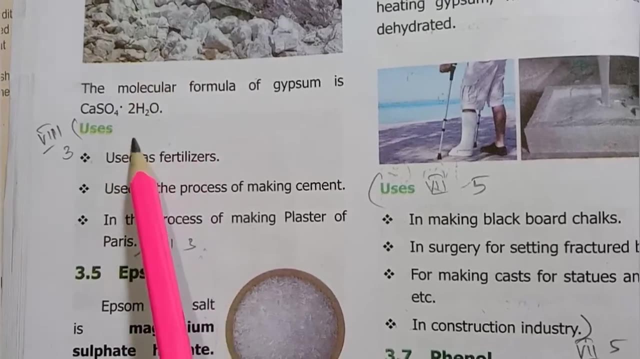 setting of cement or a close panic. only a throne letter. second one can answer. then, third one: what are the use? what are uses of gypsum, page number 40. uses of gypsum- gypsum, page number 40. the left side, left drawing cookie. the users are Kalia and the three points a throne letter. third one can answer uses of: